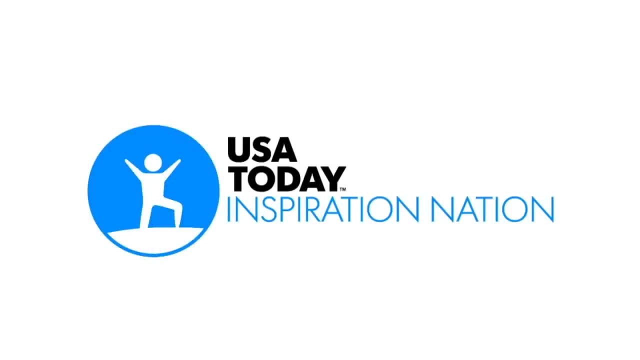 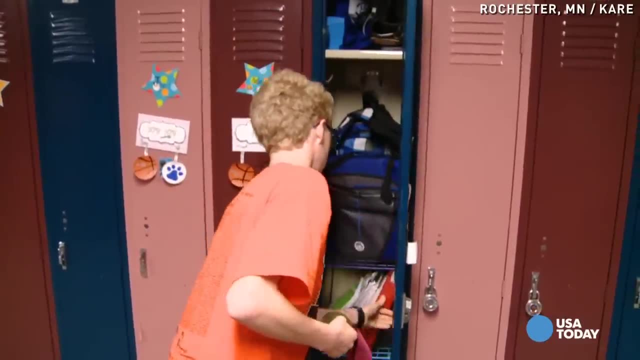 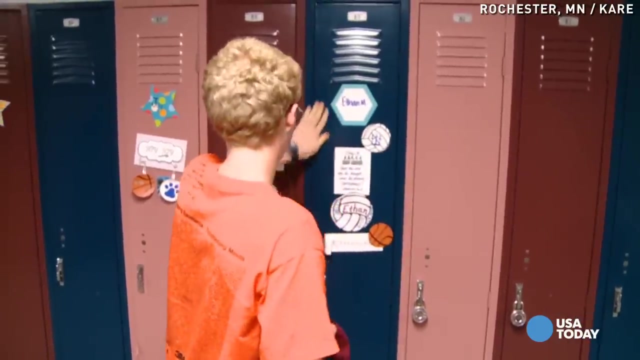 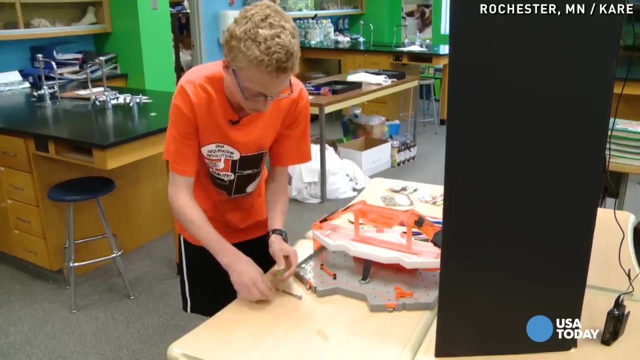 When you think scientist or major medical discovery, a 14-year-old boy fighting with his locker is probably not the mental image you conjure up, As even Ethan Manuel would admit. Yeah, really mind-blowing, But this eighth grader at Rochester Central Lutheran is behind. 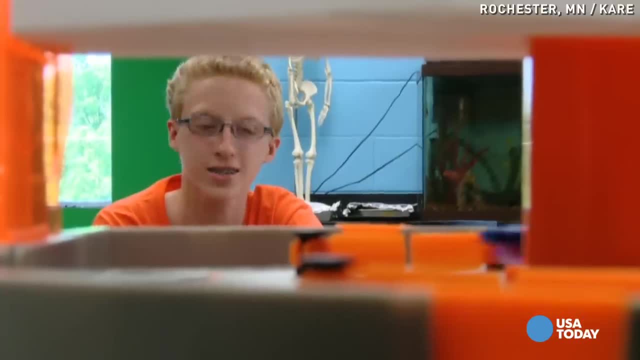 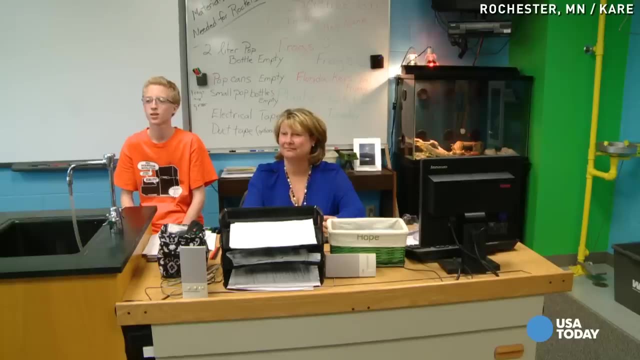 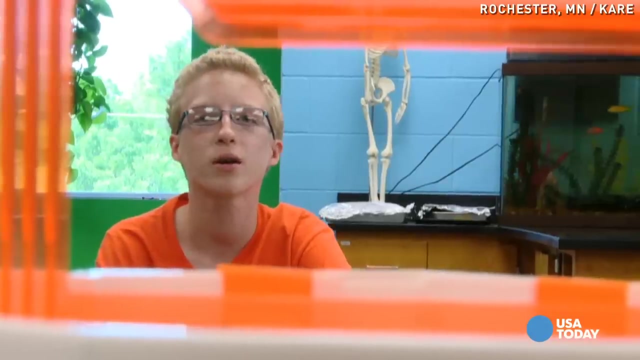 a discovery that a PhD at an academic medical mecca would be proud of. I didn't dream, or anything, that this would become like this. When Ethan's teacher, Mrs Olmland, assigned her students the task of creating a project for the school science fair, It sparked my interest a little bit, Ethan. 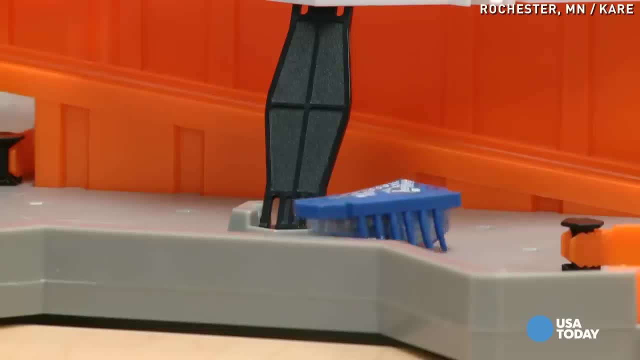 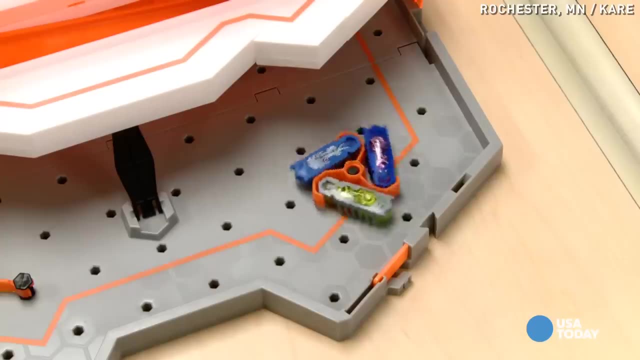 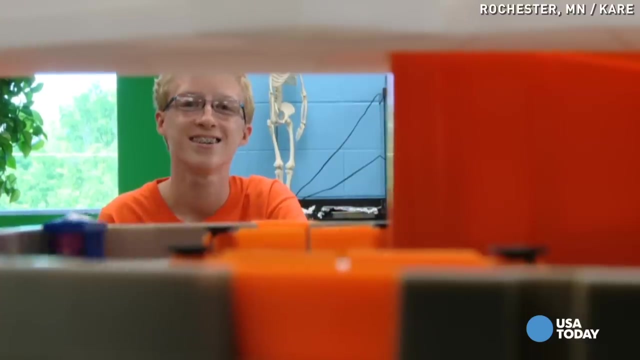 turned to his toy box. I used hex bugs, Using of all things. This is what they do: Plastic bugs. It's a robotic bug. All it does is vibrate. What he found has created a buzz loud enough to be heard, not just by Mom Leela. 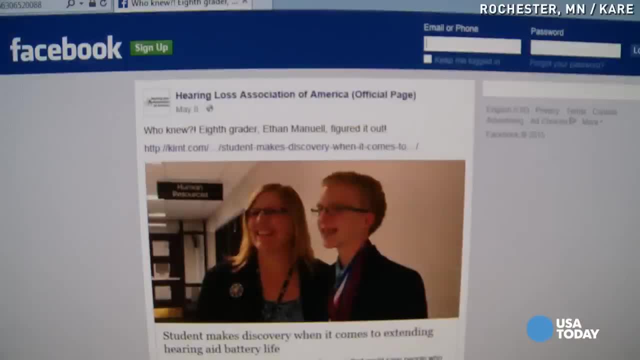 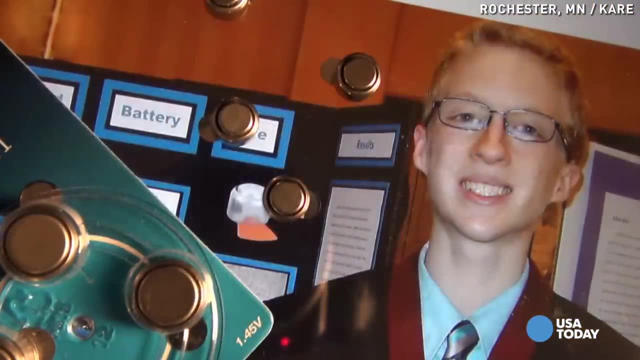 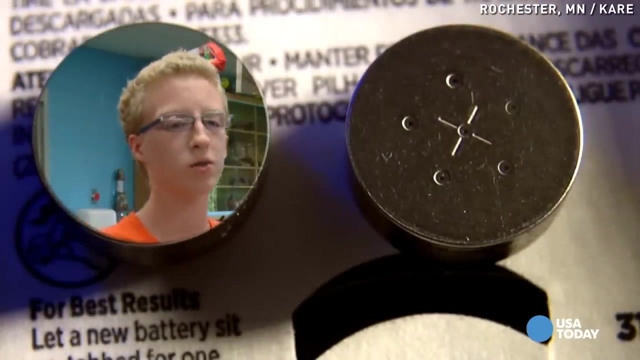 You can Google Ethan, But across cyberspace This has gone far. By converting his bugs to work with hearing aid batteries, Ethan discovered the zinc batteries last longer the longer you expose them to air before using them- With waiting five minutes, you can increase the lifespan by 85%. 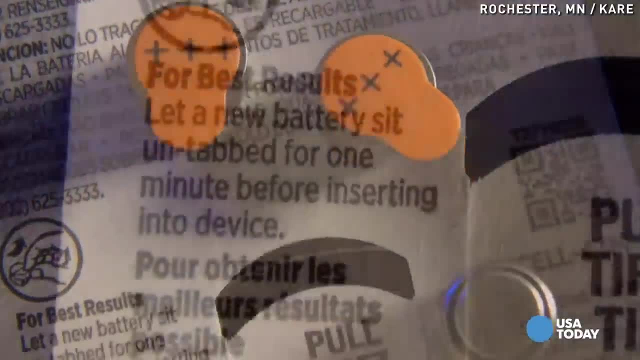 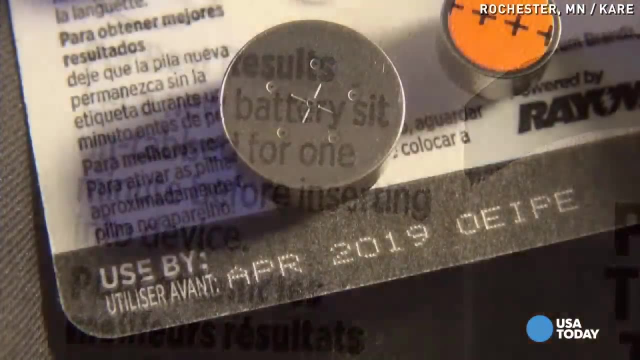 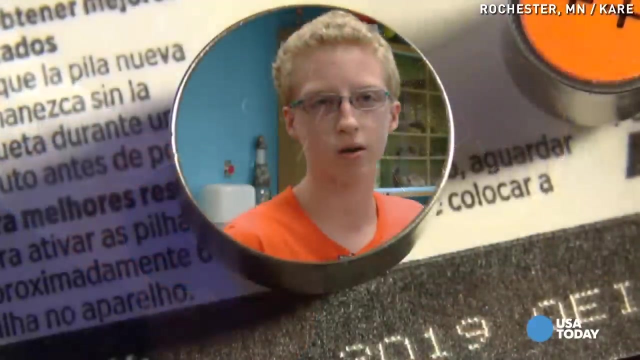 Now some hearing aid battery packets in microscopic print do warn that for the best results the battery should sit un-tabbed for one minute. Others offer no instruction at all Because most people don't know this, so they just pull the tab off and insert it Like the tab is a sticker or something, But by 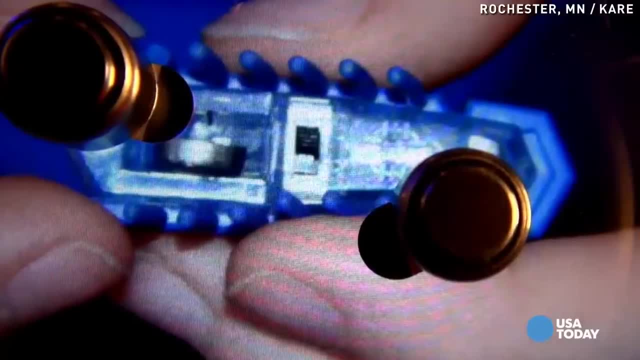 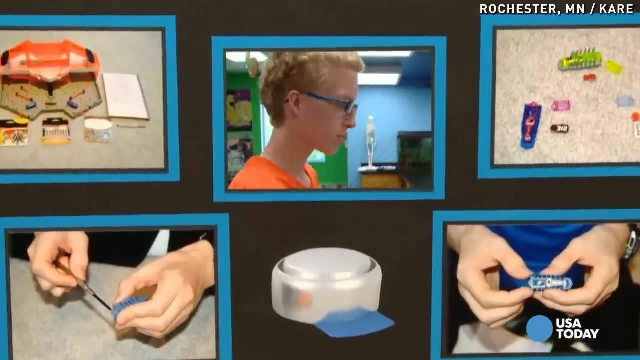 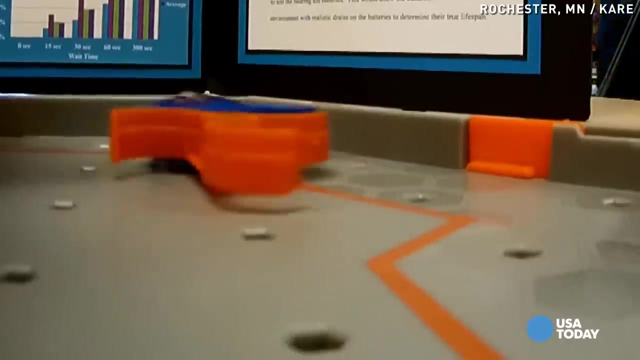 carefully monitoring how long the batteries lasted in the bugs after being left un-tabbed for various amounts of time. It's easy to tell when they're dead. they stop moving. Ethan came up with his five-minute rule: If you wait five minutes you'll get the longest battery lifespan I'm. 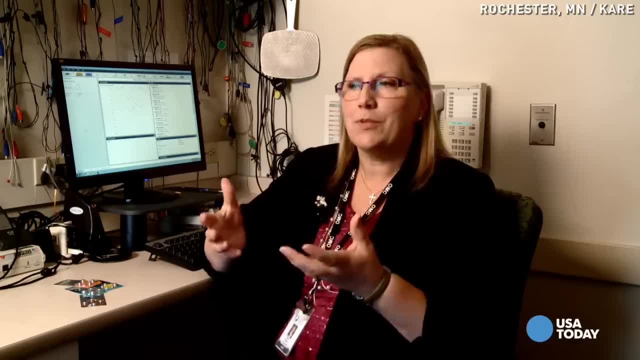 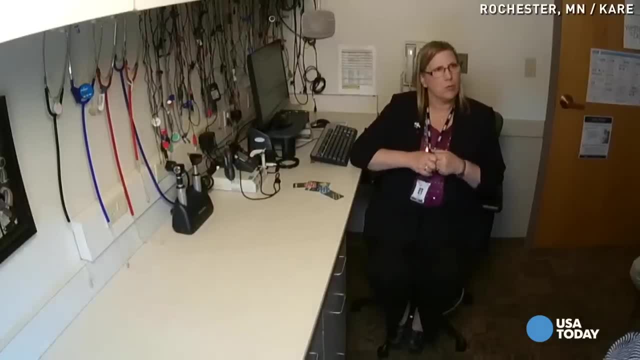 so proud of this kid Across town at Olmsted Medical Center. I keep telling my patients about it. Dr Mary Meyer and other audiologists have been using Ethan's discovery. It's in our written information when we do a fitting To help their patients save money on hearing aid batteries.